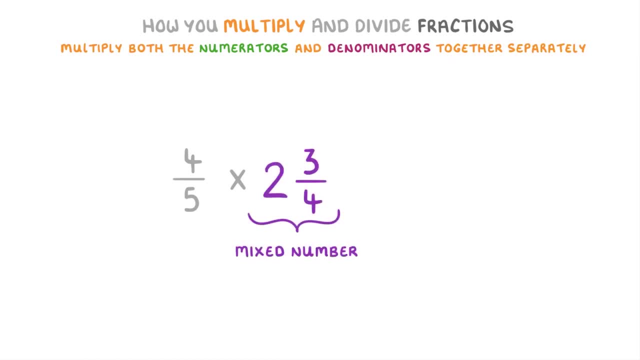 which is a mixed number. Now you can't directly multiply fractions by mixed numbers, but it's a lot easier if you take the mixed number and convert it to an improper fraction first. So to do that, we multiply the 2 by the 4 to get 8, and 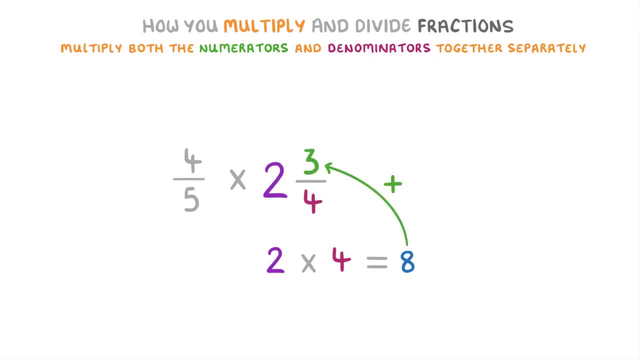 then add that 8 to the numerator of 3 to get a new numerator of 11.. So we get an improper fraction of 11 over 4.. Then we can just multiply 4 by 4 to get 4. So we get 4 fifths by 11 over 4, like in our other examples. So 4 times 11 is 44,. 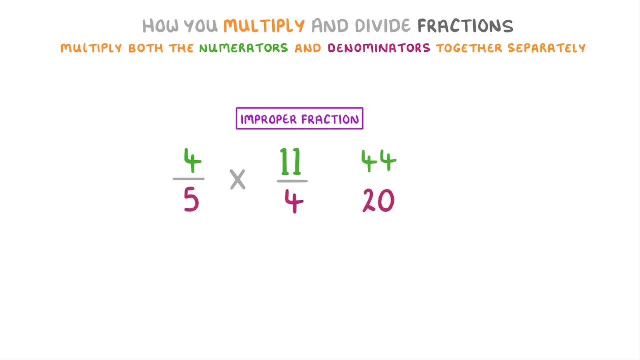 and 5 times 4 is 20, which gives us 44 over 20.. And then we can simplify that by dividing top and bottom by 4 to get 11 over 5.. One other thing to point out about multiplying fractions is that when we multiply together, 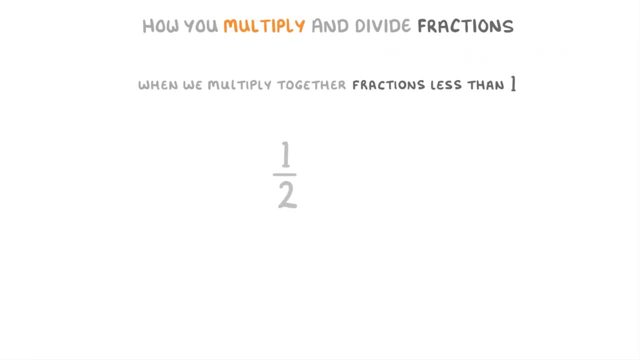 fractions that are less than or equal to 4, we get 4 over 4.. If we multiply fractions that are less than 1, like 1 half times 1 third- we actually get an even smaller number because we're taking a small portion of something that was. 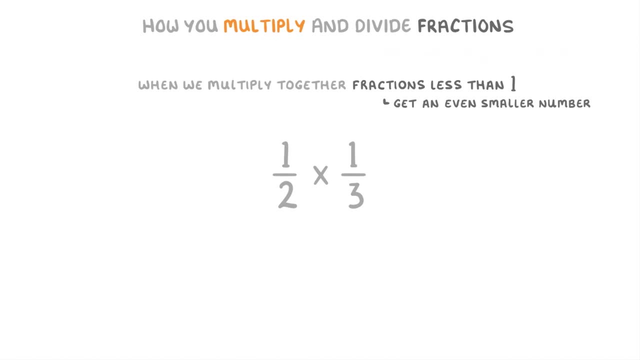 already small. For example, if we start with half a pizza, then by multiplying it by 1 third, we're effectively selecting 1 third of that half pizza. So now we only have 1 sixth of the whole pizza. In order to divide fractions, we actually use a trick. First of all, you want to write. 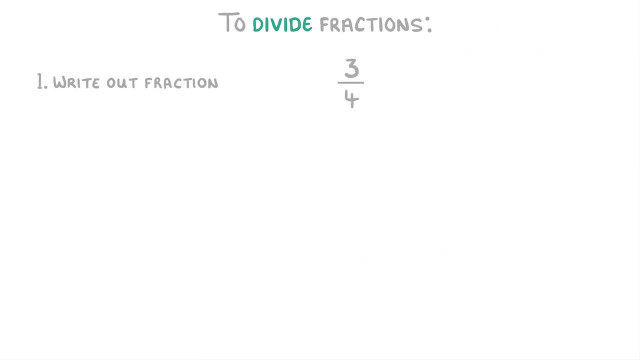 out the fraction, For example 3 quarters divided by 5 ninths. Then you flip the second fraction upside down, So change the 5 over 9 to 9 over 5. And then we can rewrite the question with a multiply. 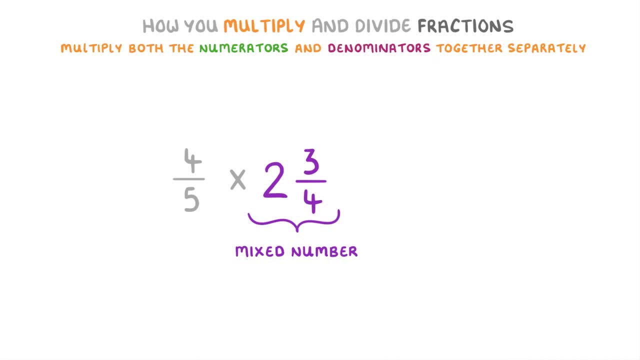 numbers. but it's a lot easier if you take the mixed number and convert it to an improper fraction first. So to do that, we multiply the 2 by the 4 to get 8, and then add that 8 to the numerator of 3 to get a new numerator of 11.. So we get an. 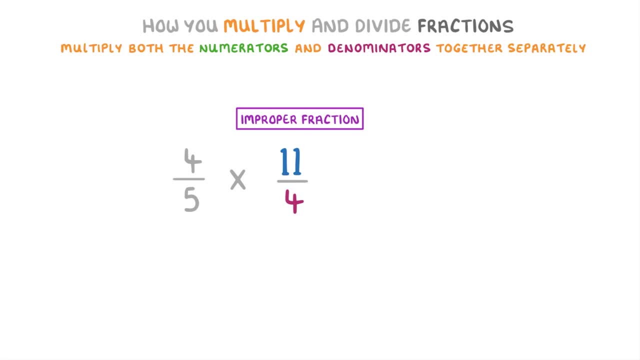 improper fraction of 11 over 4.. Then we can just multiply 4 by 4 to get 4.. So we get 4 fifths by 11 over 4, like in our other examples. So 4 times 11 is 44,. 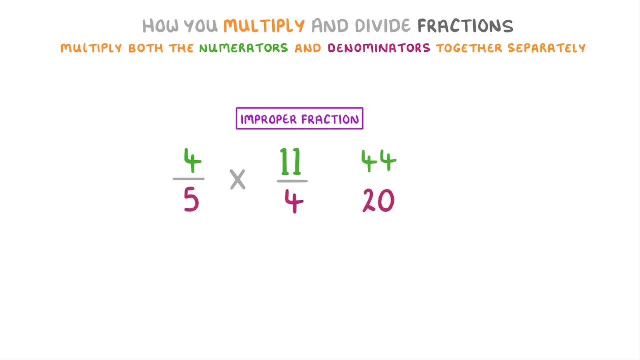 and 5 times 4 is 20, which gives us 44 over 20.. And then we can simplify that by dividing top and bottom by 4 to get 11 over 5.. One other thing to point out about multiplying fractions is that when we multiply together, 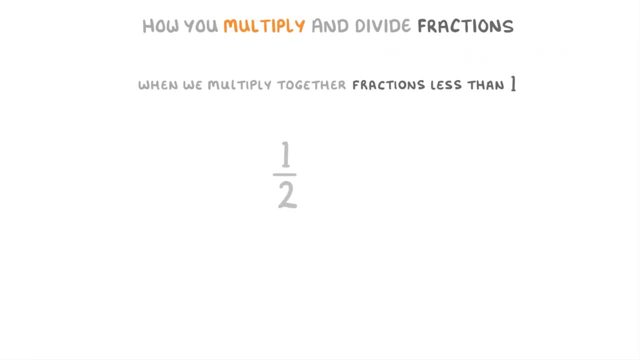 fractions that are less than or equal to 4, we get 4 over 4.. If we multiply fractions that are less than 1, like 1 half times 1 third- we actually get an even smaller number because we're taking a small portion of something that was. 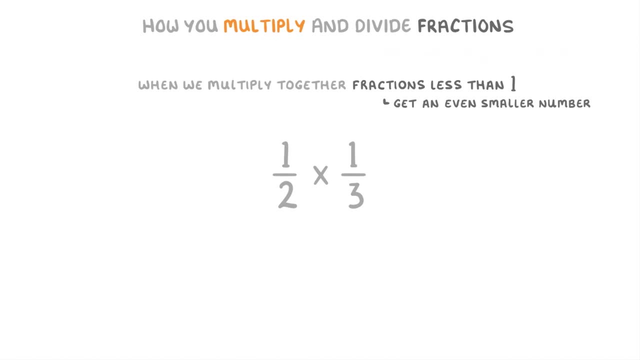 already small. For example, if we start with half a pizza, then by multiplying it by 1 third, we're effectively selecting 1 third of that half pizza. So now we only have 1 sixth of the whole pizza. In order to divide fractions, we actually use a trick. First of all, you want to write. 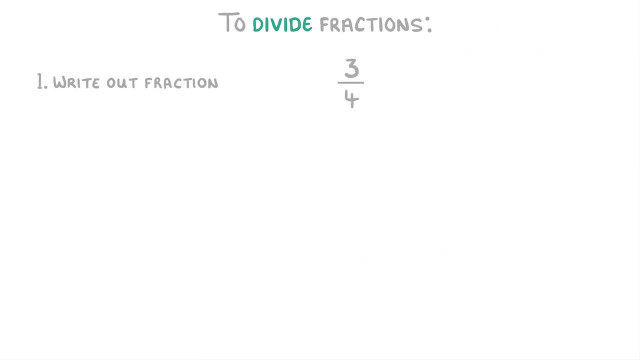 out the fraction, For example 3 quarters divided by 5 ninths. Then you flip the second fraction upside down, So change the 5 over 9 to 9 over 5. And then we can rewrite the question with a multiply. 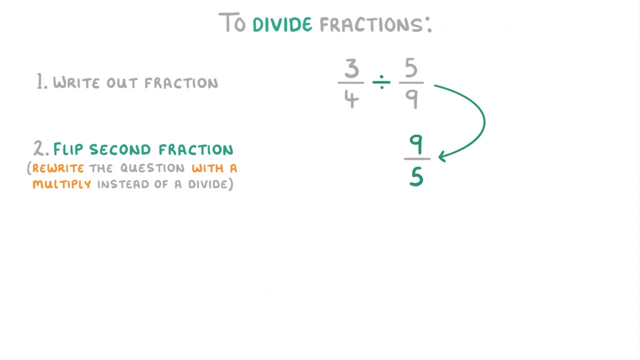 Multiply instead of a divide, which means that we'll have 3 quarters times 9 fifths. So all we've done is flip the second fraction upside down and change the divide to a multiply. Then we can just multiply the fractions together as usual. So here we're to do 3 times 9 to 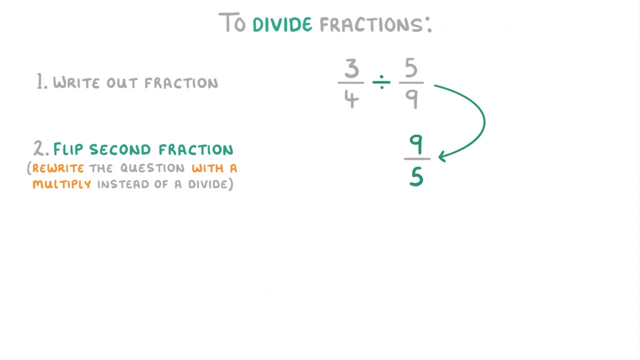 Multiply instead of a divide, which means that we'll have 3 quarters times 9 fifths. So all we've done is flip the second fraction upside down and change the divide to a multiply. Then we can just multiply the fractions together as usual. So here we're to do 3 times 9 to 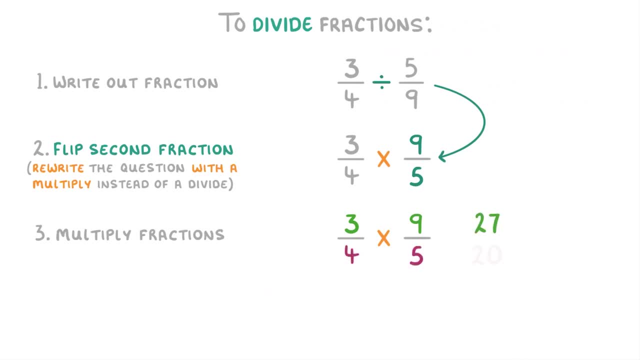 give us 27, and 4 times 5 to give us 20.. So we have 27 over 20.. And as a last step, we need to check if it can be simplified, Which it can't. So the answer stays as 27 over 20.. 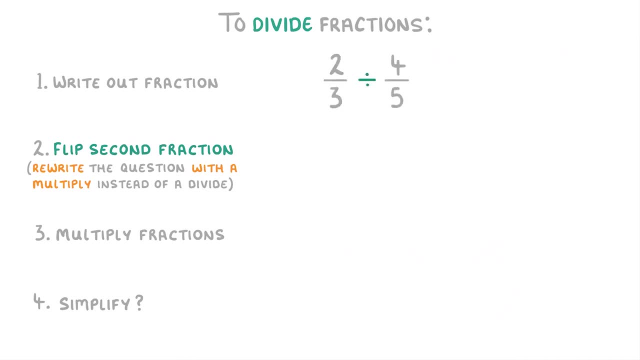 Let's try a couple more. In this one we're dividing 2 thirds by 4 fifths. So we flip the 4 fifths upside down to make it 5 over 4. And then change the divide to a multiply. 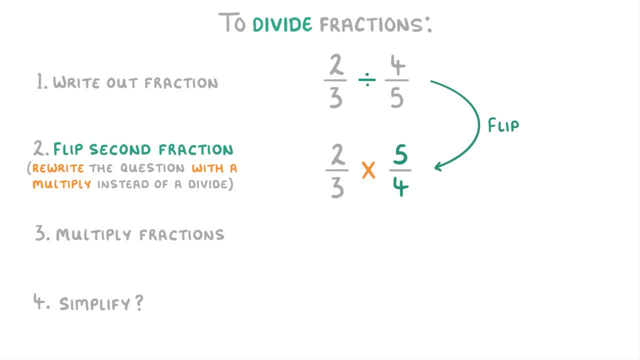 So that we can multiply them like normal: 2 times 5 is 10, and 3 times 4 is 12.. So we have 10 over 12. Which we can simplify by dividing top and bottom by 2, to get 5 over 6.. 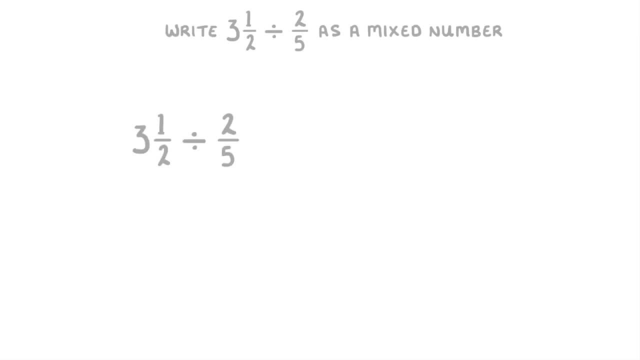 In this question we're dividing 3 and a half by 2 fifths. The fact that we need the answer in the form of a mixed number doesn't change how we do the question at all. It just means that we're going to have to convert it into mixed number. 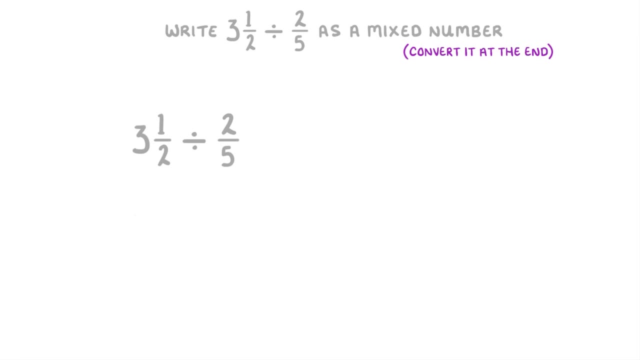 form at the end. The first step, though, is to convert this 3 and a half, which is a mixed number, into an improper fraction, to make things easier for ourselves. So we do 3 times 2, which is 6.. 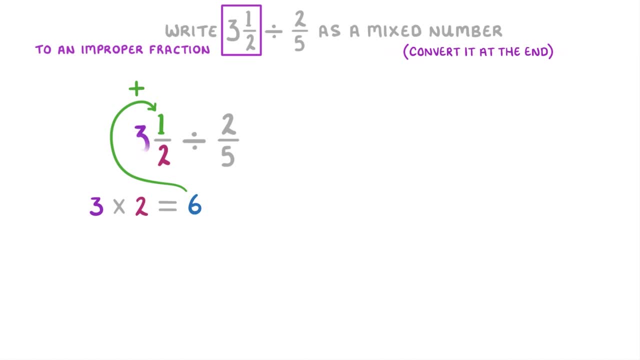 And then add that to the numerator. So because 6 plus 1 is 7,, we end up with 7 over 2.. And our question now reads: 7 over 2, divided by 2 over 5.. Then, like always, we flip the 2 over 5 upside down to get 5 over 2.. 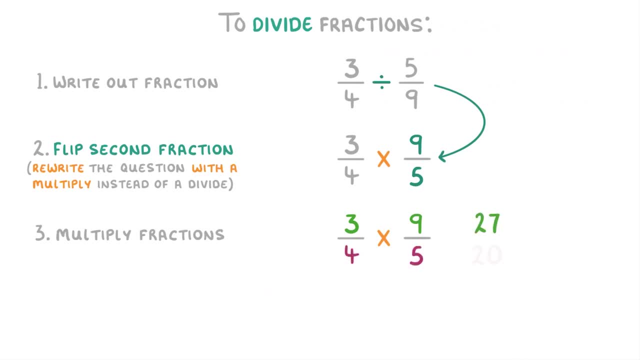 give us 27, and 4 times 5 to give us 20.. So we have 27 over 20.. And as a last step, we need to check if it can be simplified, Which it can't. So the answer stays as 27 over 20.. 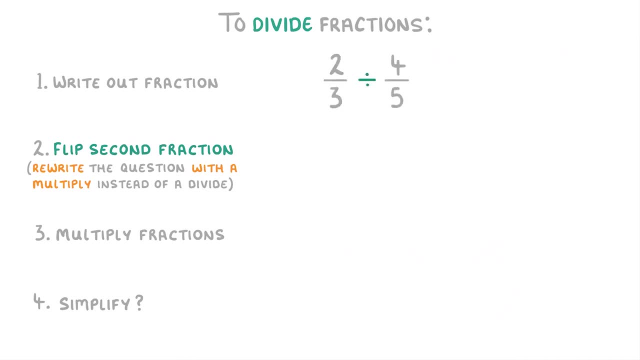 Let's try a couple more. In this one we're dividing 2 thirds by 4 fifths. So we flip the 4 fifths upside down to make it 5 over 4. And then change the divide to a multiply. 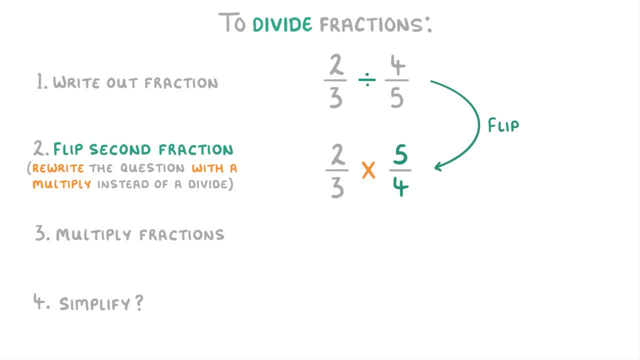 So that we can multiply them like normal: 2 times 5 is 10. And 3 times 4 is 12.. So we have 10 over 12.. Which we can simplify by dividing top and bottom by 2, to get 5 over 6.. 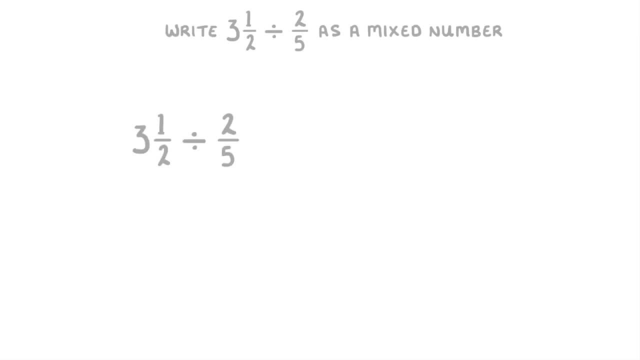 In this question we're dividing 3 and a half by 2 fifths. The fact that we need the answer in the form of a mixed number doesn't change how we do the question at all. It just means that we're going to have to convert it into mixed number. 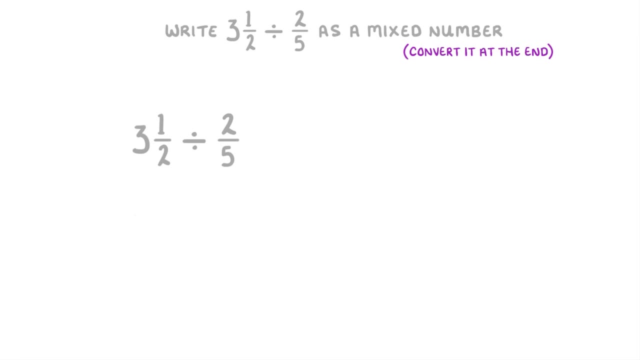 form at the end. The first step, though, is to convert this 3 and a half, which is a mixed number, into an improper fraction, to make things easier for ourselves. So we do 3 times 2, which is 6.. 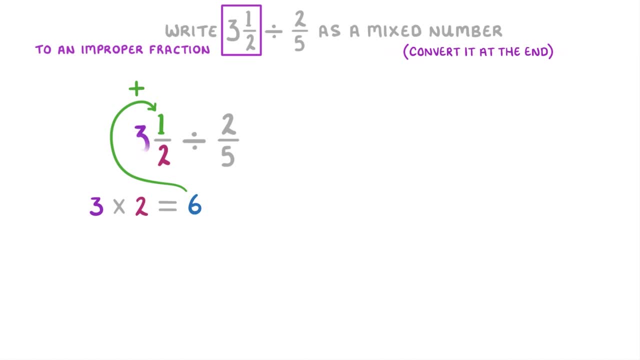 And then add that to the numerator. So because 6 plus 1 is 7,, we end up with 7 over 2.. And our question now reads: 7 over 2, divided by 2 over 5.. Then, like always, we flip the 2 over 5 upside down to get 5 over 2.. 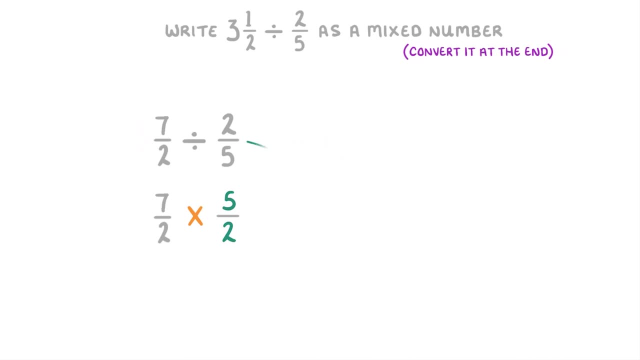 And change the divide to a multiply. So we're going to have to do 7 over 2.. 7 times 5,, which is 35. And 2 times 2,, which is 4. To get 35 over 4..